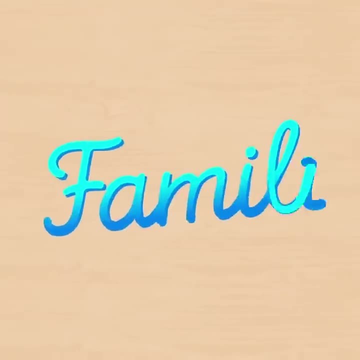 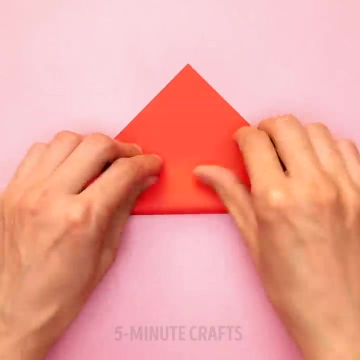 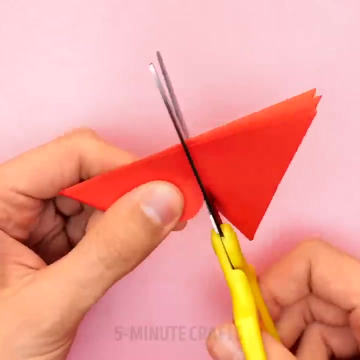 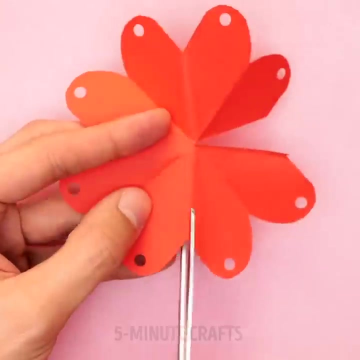 I can feel my body cold against the concrete, but I can't seem to get enough. My mind is fixed on what it wants. I just let you beat me. Looks can be deceiving. Let you get the best of me In bed with my worst enemy. This is a no-go. I just can't take hold. This is a danger zone. 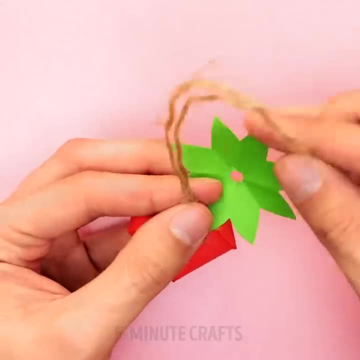 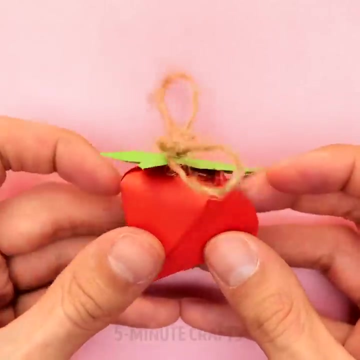 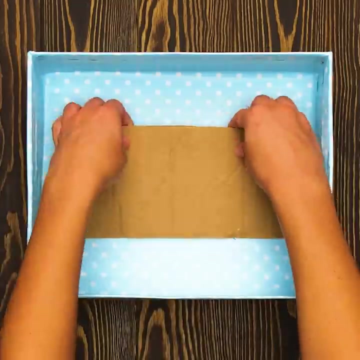 Pack up and get me home. This is a no-go. I just can't take hold. This is a danger zone. Pack up and get me home, Hand in mine, Follow me. Let me waste your time. Sit up, eat, do some stupid shit. Take a seat. Let me waste your time. Throw off these supper chow, Supper chow, You be the fastest%. Turn all of me up. Treat you like you're heaven. Thought that I knew better. Keep falling for your Innocence, Acting like you're into me. 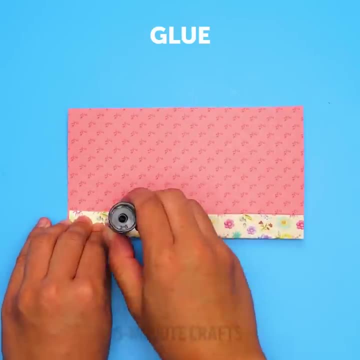 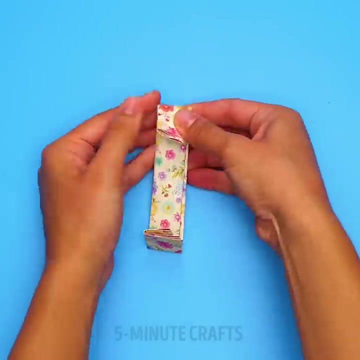 I know this is hopeless. Moving in slow motion externally Climate doesn't fit Too if it's going withα magnet. There's a want? get rid of You. do tend on me. This is a no-go. No sex, So all my machines will be gone. 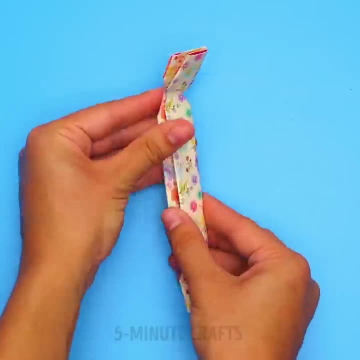 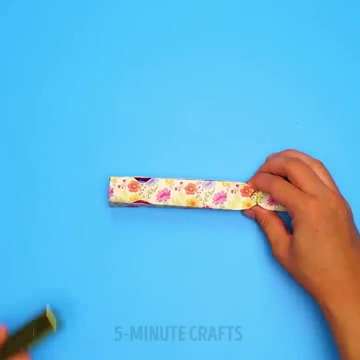 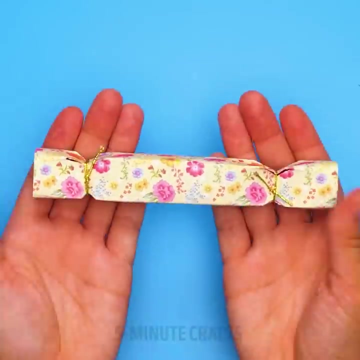 Can she get up It? If no, ASAP. Oh, this is the danger zone. Back up and get me. So put your hand in mine, Follow me. Let me waste your time. Stella B, Do some stupid shit. Take a seat. Let me waste your time. 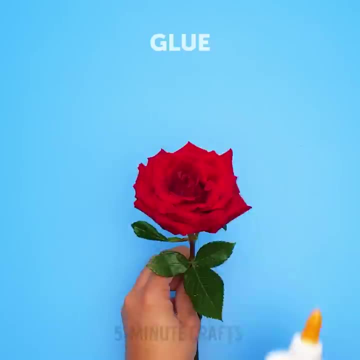 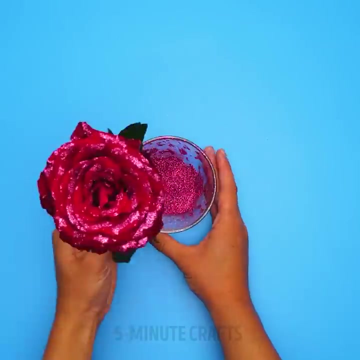 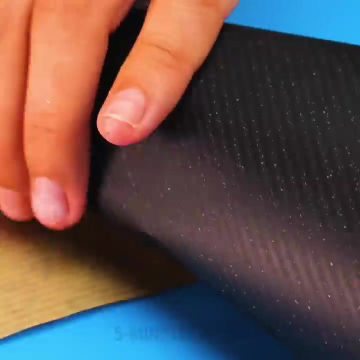 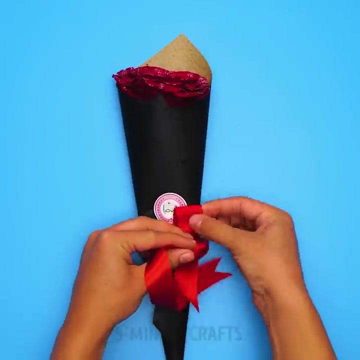 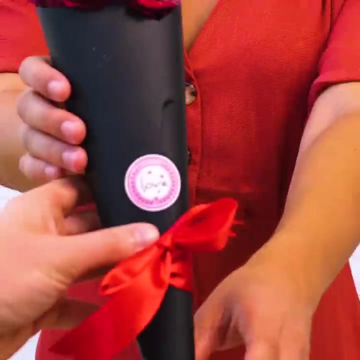 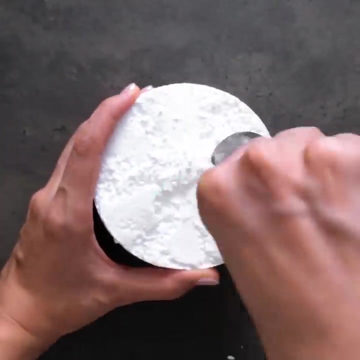 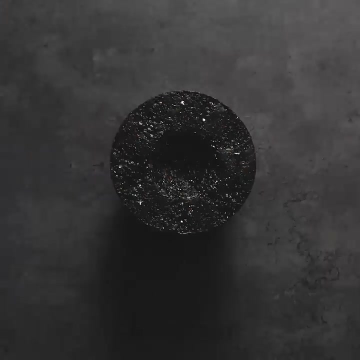 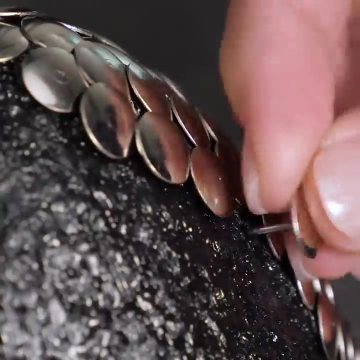 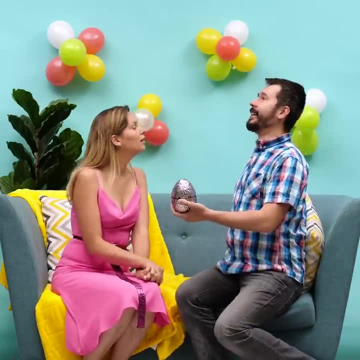 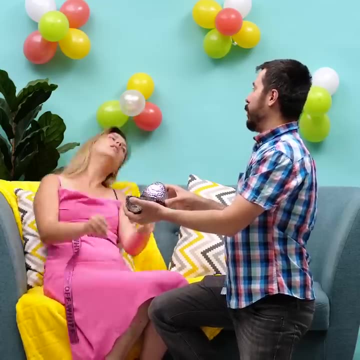 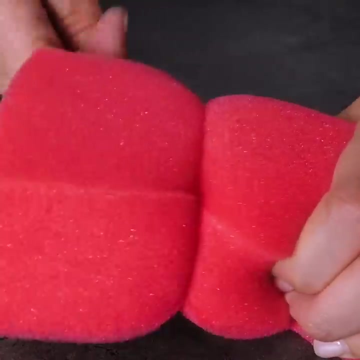 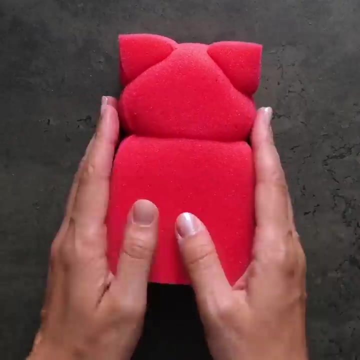 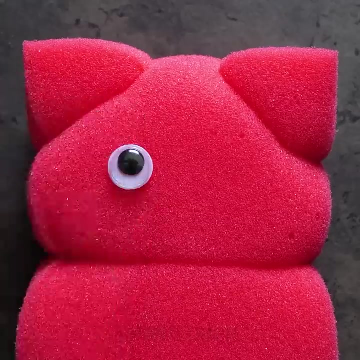 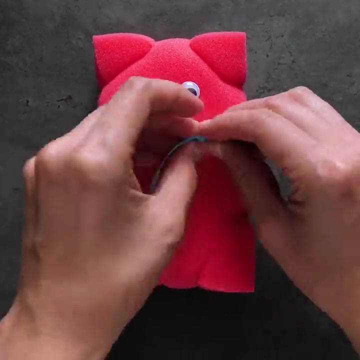 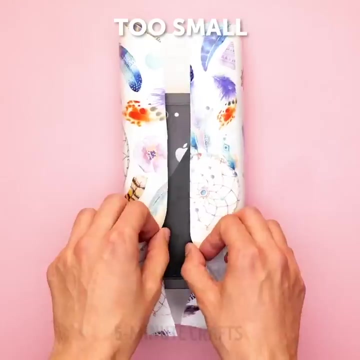 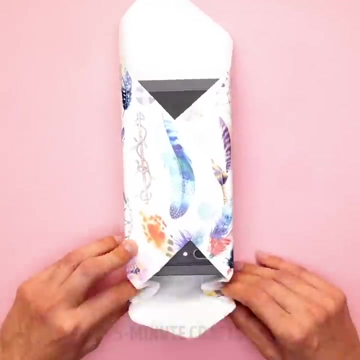 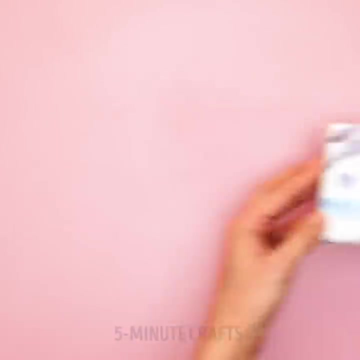 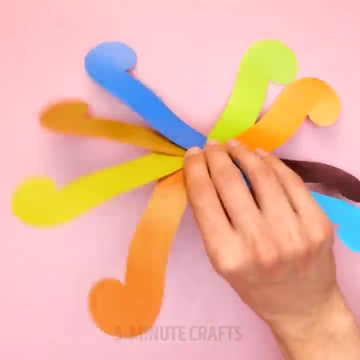 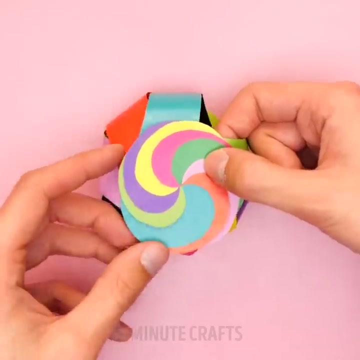 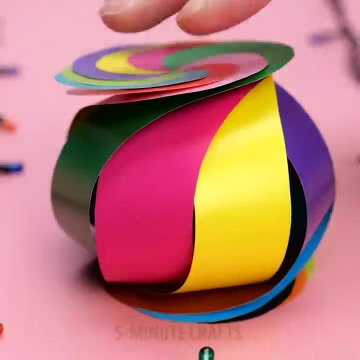 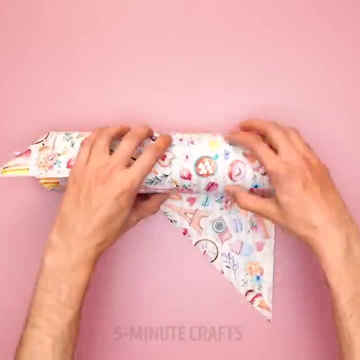 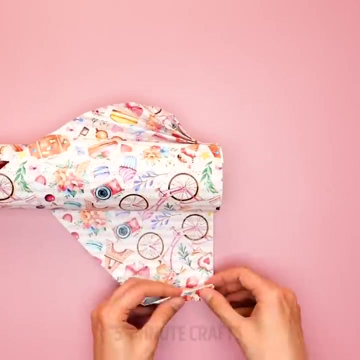 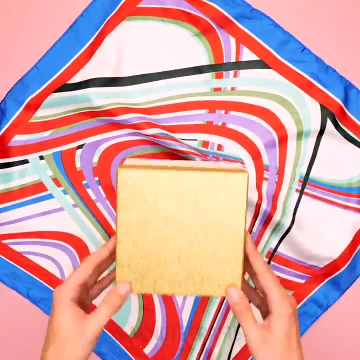 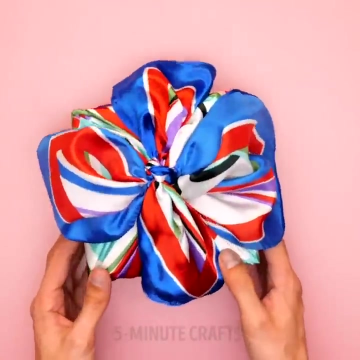 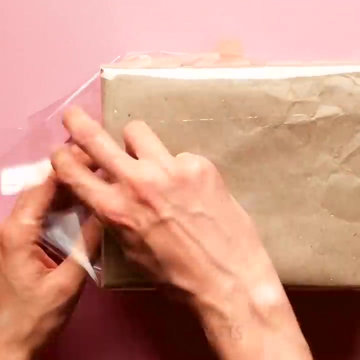 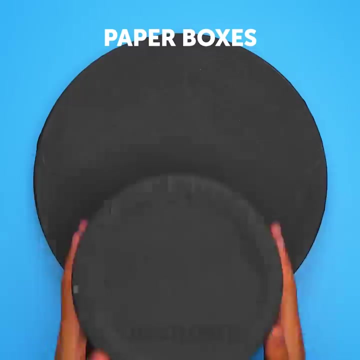 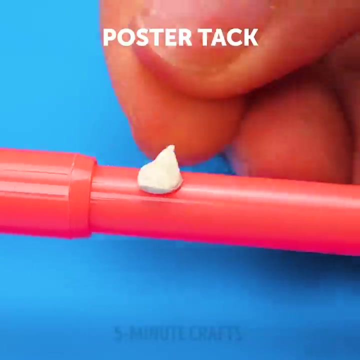 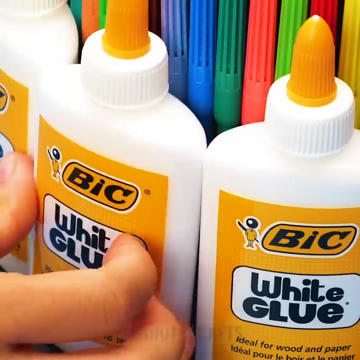 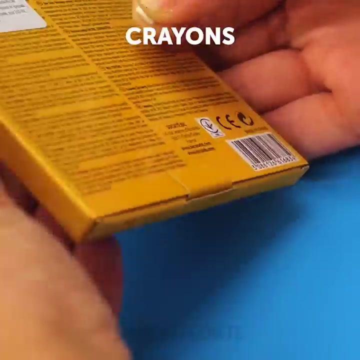 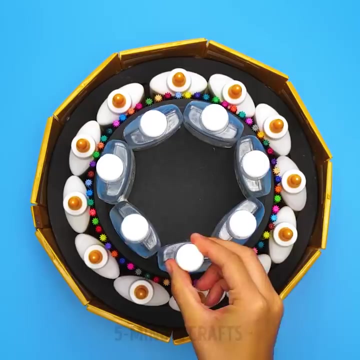 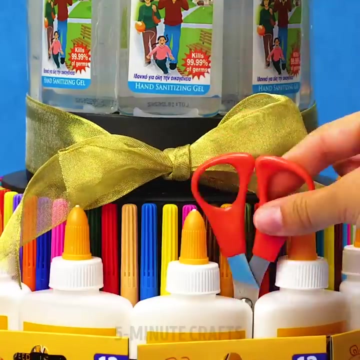 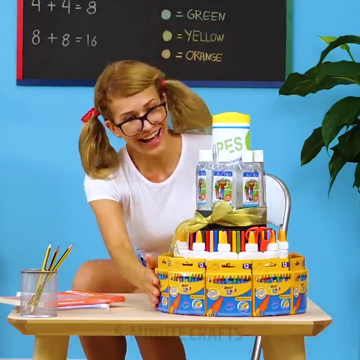 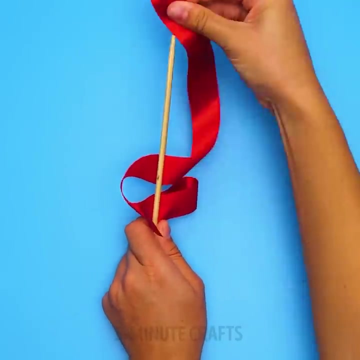 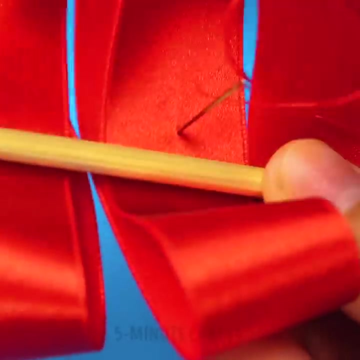 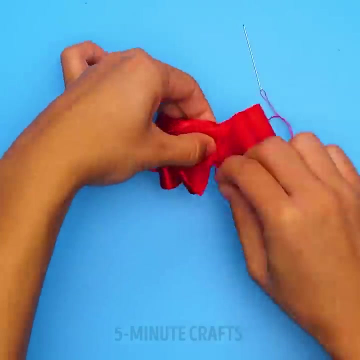 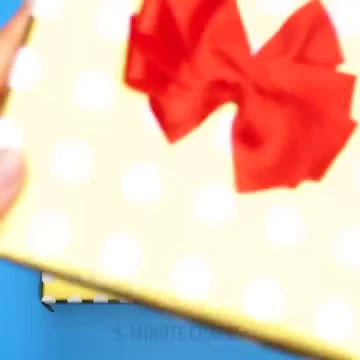 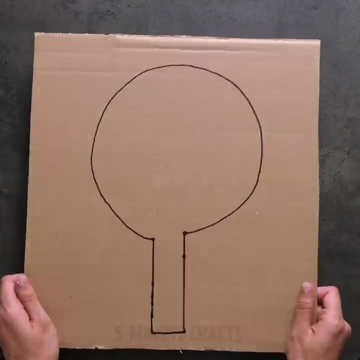 Look at me. I'm in a bad situation. Look at him. he's got a bad reputation. They've been looking at us. Why do I need to be good all the time? I'm wrapped around his finger, but he is mine. 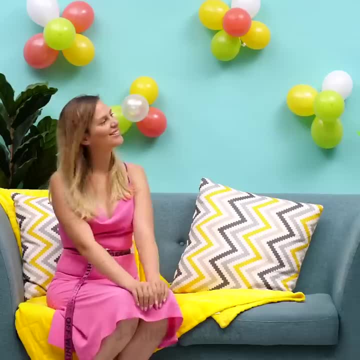 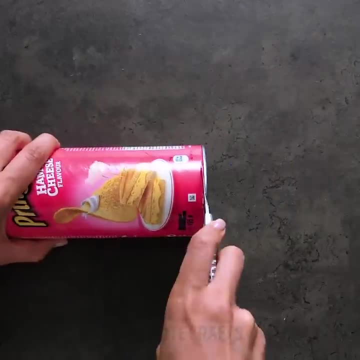 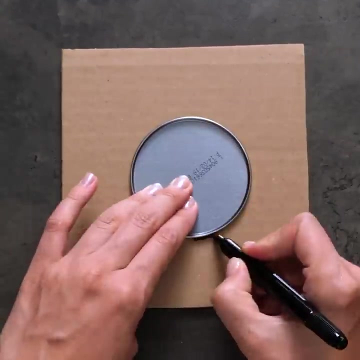 Don't care what they say, too late anyway. Why do I need to be good all the time? Yeah, it gets. when I'm in a bad mood, Then he, he knows how to make it all right. Yeah, I get that. he got a history. 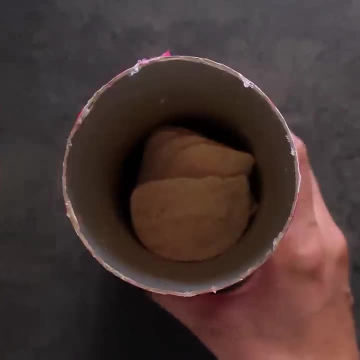 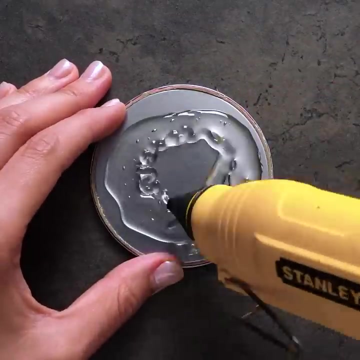 But I don't want to think about no other than us. They look at me, I'm in a bad situation. Look at him, he's got a bad reputation. They've been looking at us, thinking we are too much. Look at me, I'm in a bad situation. 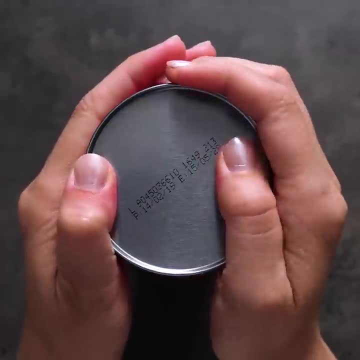 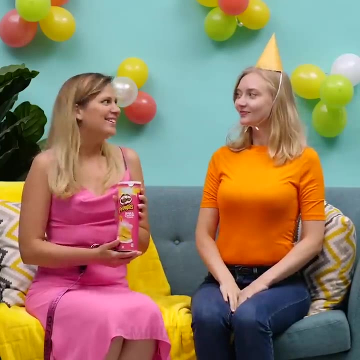 Look at him. he's got a bad reputation. They've been looking at us, thinking we are too much. Look at me. I'm in a bad situation. Why do I need to be good all the time? I'm wrapped around his finger, but he is mine. 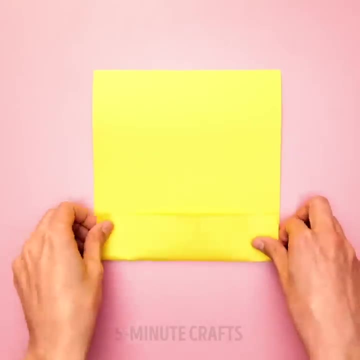 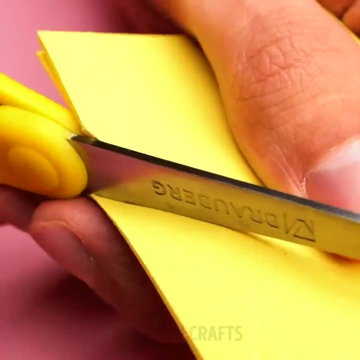 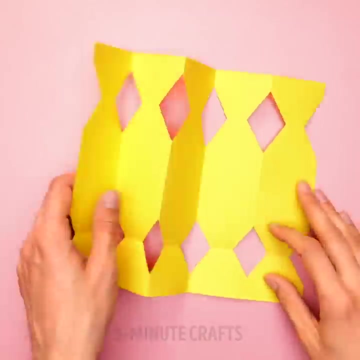 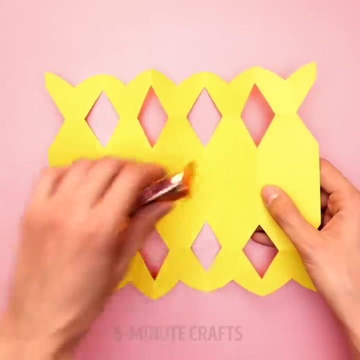 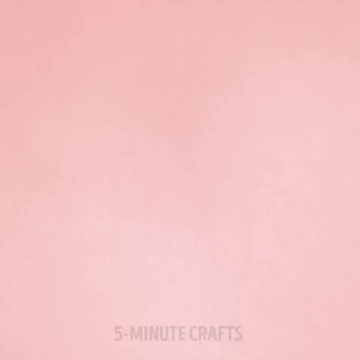 Don't care what they say, too late anyway. Why do I need to be good all the time? Nah, nah, nah, No drama, no drama. yeah, Nah, nah, nah, No drama. He's got a bad history, but what about it? 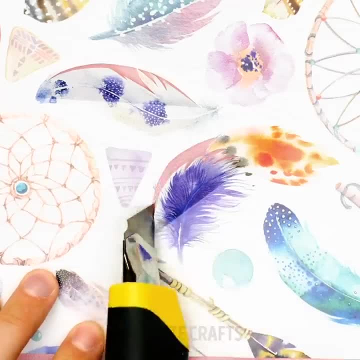 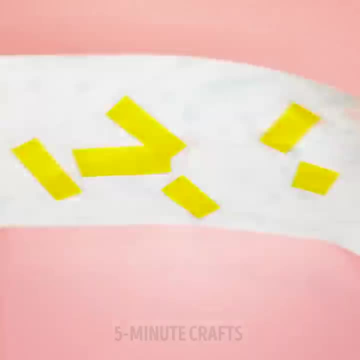 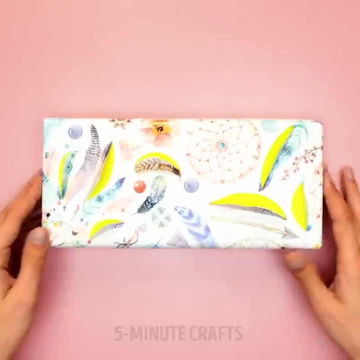 Yeah, he's got a bad history, but I want him anyway. So look at me, I'm in a bad situation. Look at him, he's got a bad reputation. But what about it? Why do I need to be good all the time? 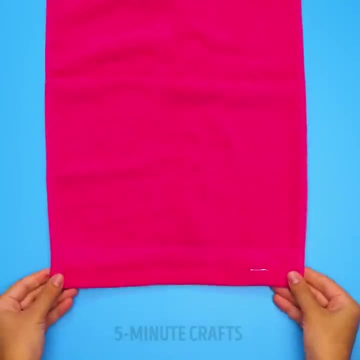 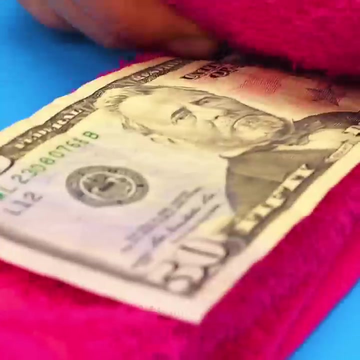 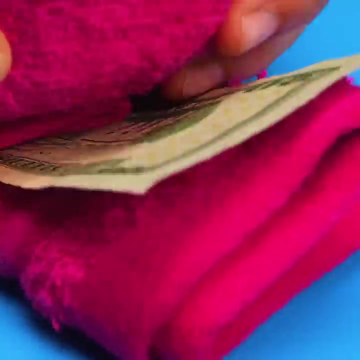 I'm wrapped around his finger, but he is mine, Don't care what they say. too late anyway. Why do I need to be good all the time? Nah, nah, nah, no drama, no drama. yeah, Nah, nah, nah, no drama, no drama, yeah. 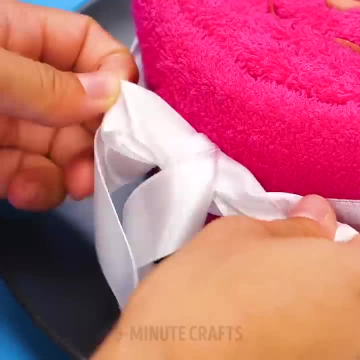 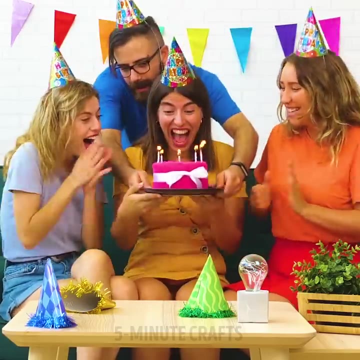 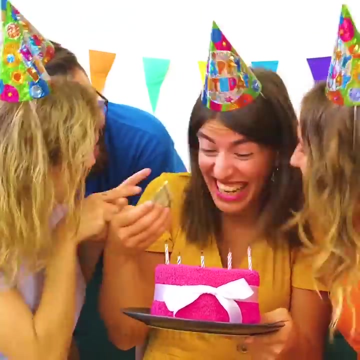 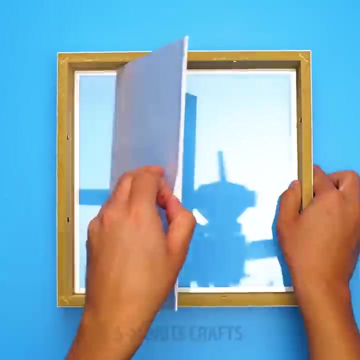 Nah, nah, Nah, nah, nah, no drama, no drama. yeah, Nah, nah, nah, no drama, no drama. yeah, yeah, I see a sky with a rain. you're caught, but I'm not runnin'. I see it danglein' all too fast, but I'm not leavin'. 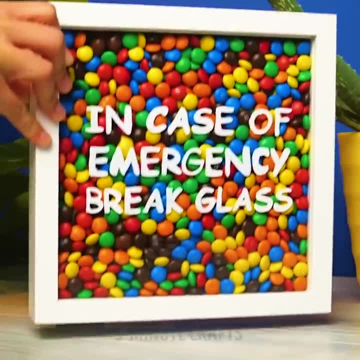 I see it danglein' all too fast, but I'm not leavin'. I see it danglein' all too fast but I'm not leavin', And you go round and round and round and you cannot see. I'll go right behind you, I'll be the tree. 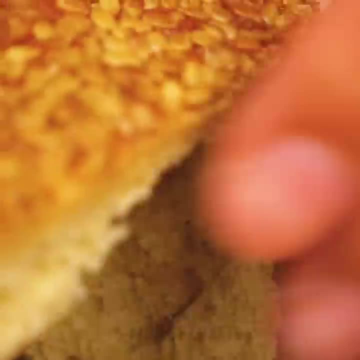 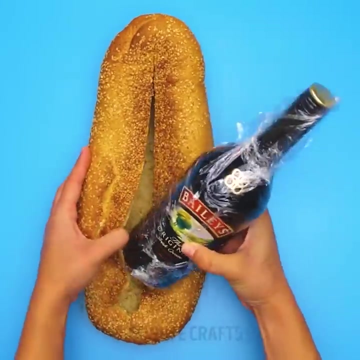 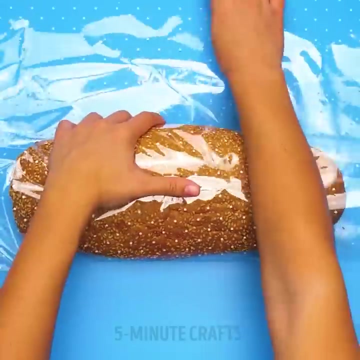 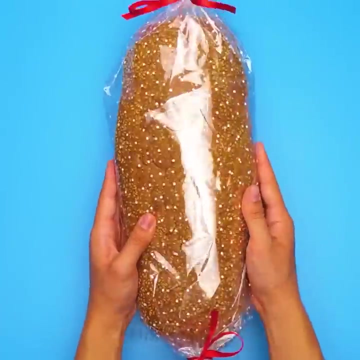 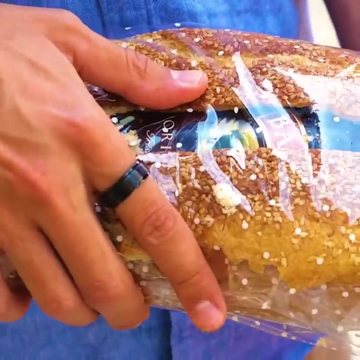 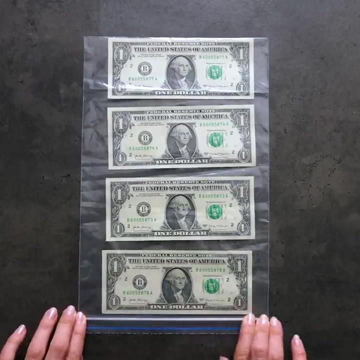 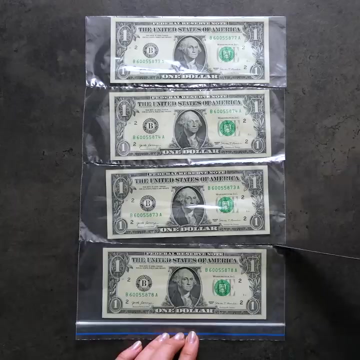 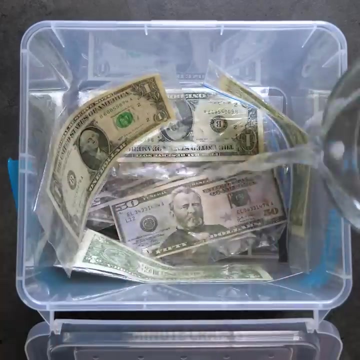 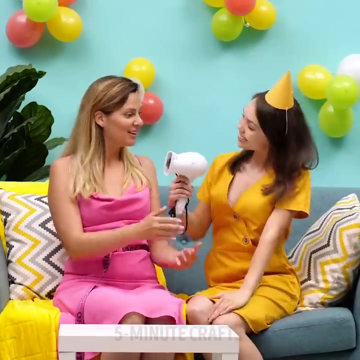 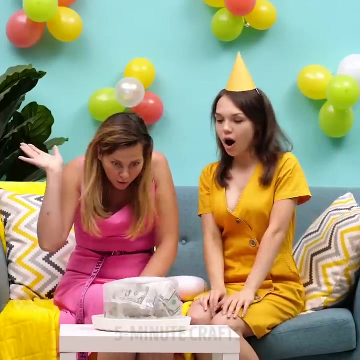 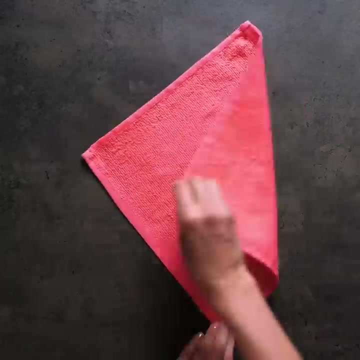 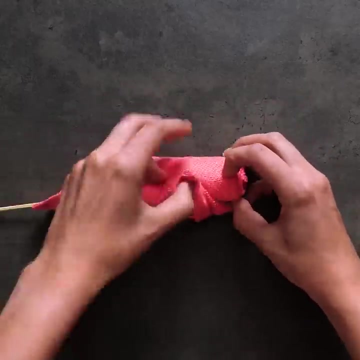 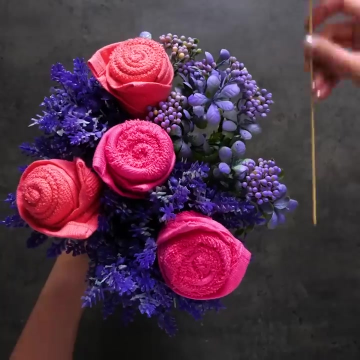 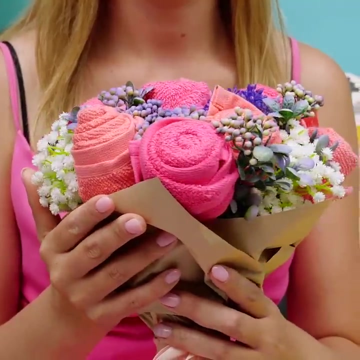 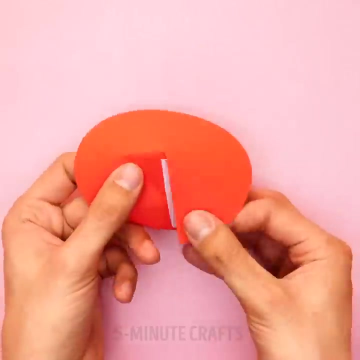 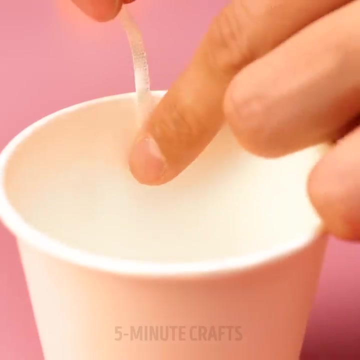 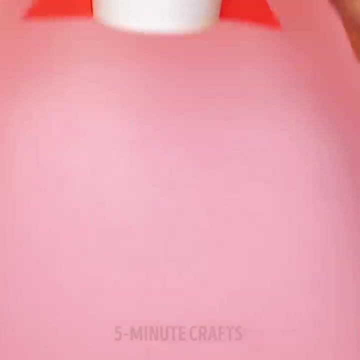 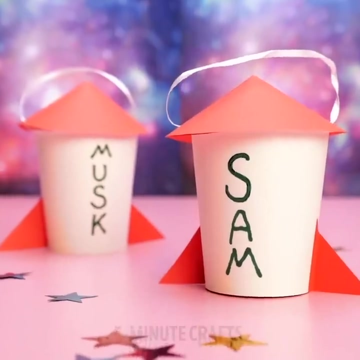 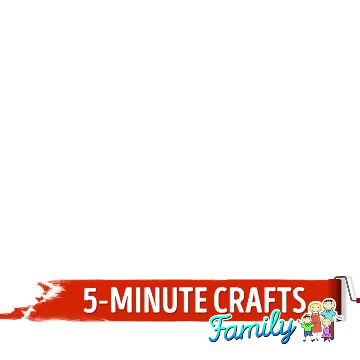